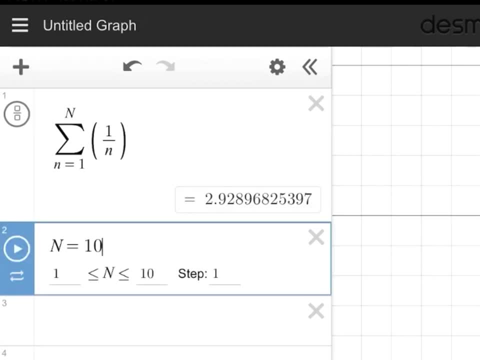 Now let's include lots and lots of terms. I'm going to go up to here and just start adding zeros. Let's do the first 100 terms added together and notice we get 5.18.. The first thousand terms added together: 7.48.. The first 10,000 terms added together: 9.78. 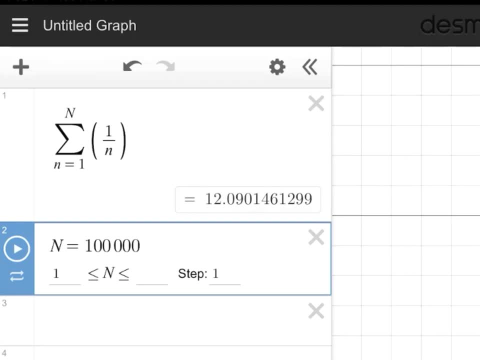 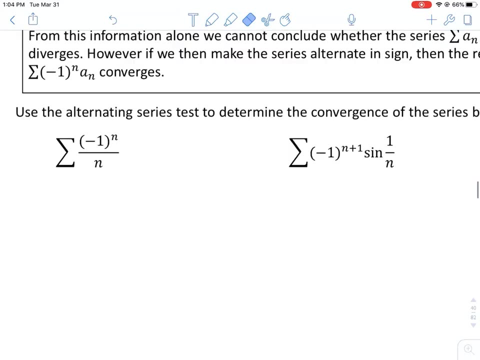 A hundred thousand terms added together, Notice, the sum keeps going up. Now it's not going up a lot, but it keeps going up and doesn't seem to stabilize. Let's go back to our notes and I want to explore this little series. you see, right here I'm going to put it: n equals one, as 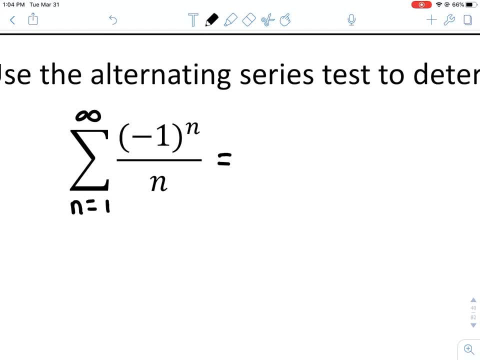 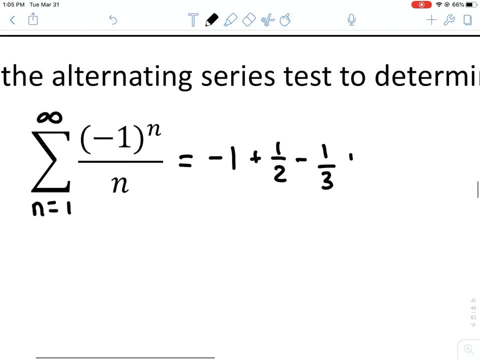 a starting value and go up to infinity. Plug in one for n first. Plug in n equals two, Plug in n equals three. So we just get negative one third. Plug in a four, You're going to get positive one fourth. Notice, we're just going to get alternating signs and otherwise it looks like the harmonic. 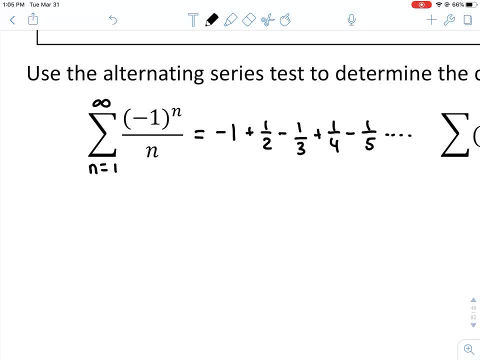 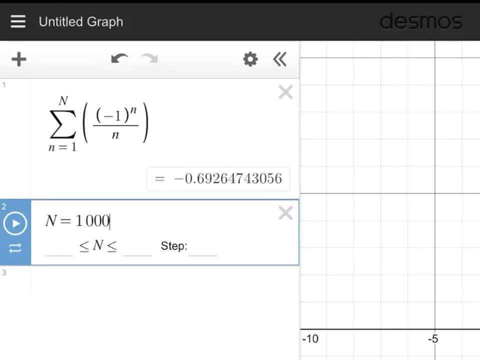 series, but some of the terms are now negative. Let's explore this one in Desmos. Okay, there's the sum of the first 10 terms, the first hundred terms. First thousand terms, First 10,000 terms, Hundred thousand terms. Well, look at the sum. It looks. 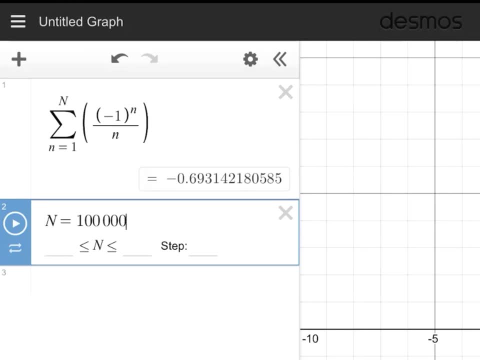 like, the sum is stabilizing at around negative 0.693.. This is an indication that we're looking at a convergent series. Adding up, all the terms of this series appear to be equal to a certain finite number. What if I wanted to make it so that the first term is positive, then negative? 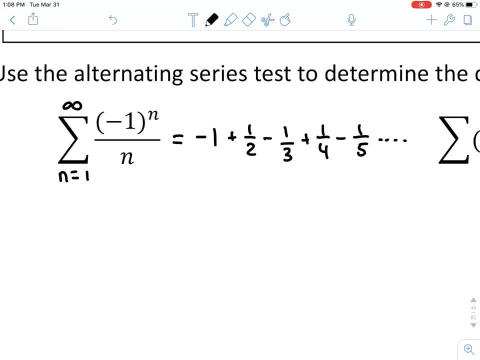 then positive, then negative, then positive. One way you could do this would be to do a series To get the negatives and positives switched. just offset the power by one and leave everything else the same. Test this out: Plug in n equals one. Now we're looking at negative. one squared, That's positive. 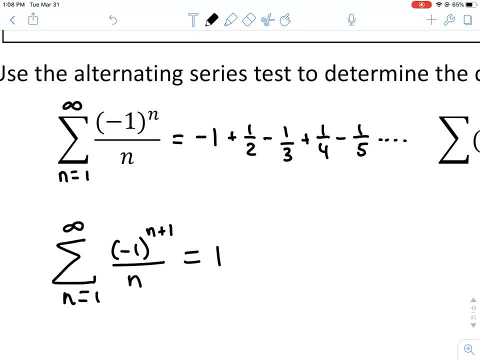 one over one, So we actually had a positive one to start. Then plug in n equals two. You're going to wind up getting a negative one half, and then you're going to get a positive one, third, negative one, fourth. So this is the harmonic series that's alternating in sign, starting with a positive one. 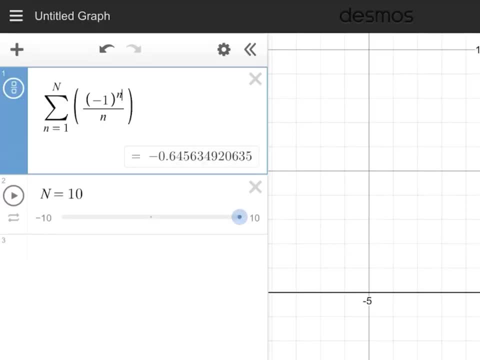 this time Let's use Desmos to figure out what's going on here. Let me put parentheses on that and say n plus one. Here's the sum of the first 10 terms of the series 0.645.. The sum of the first. 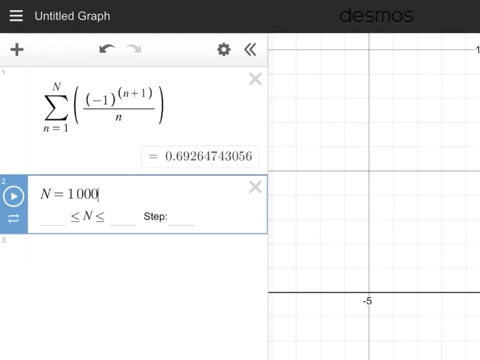 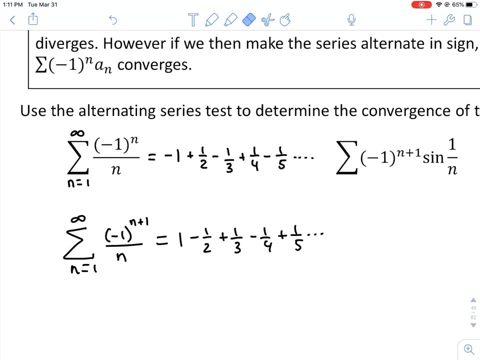 100 terms: 0.688.. 1,000 terms: 0.6926.. 100,000 terms: 0.693.. I'm getting stabilization again. All right In both cases, whether the alternating was negative, positive. 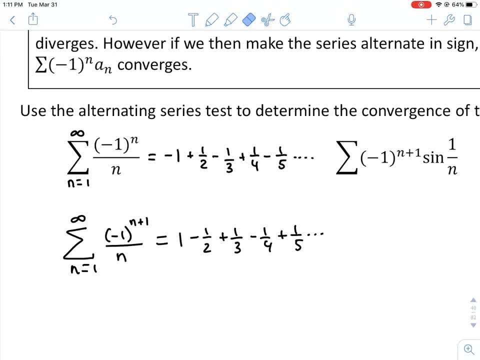 negative or positive, negative, positive, as long as it was alternating. it appears that we get convergent sums, So this one turned out to be approximately negative: 0.69.. And this one turns out to be approximately positive: 0.69.. Yet if I don't have alternating, 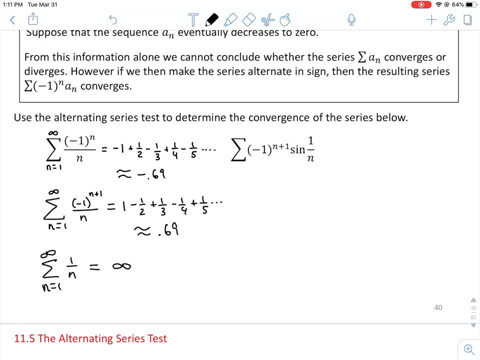 we get infinity, We have a divergent series. All of this is a lead up to a realization: that when you do have terms that shrink to zero and then you add them all up, there's no guarantee that you're going to get a finite number. However, it turns out that if you have terms that shrink to 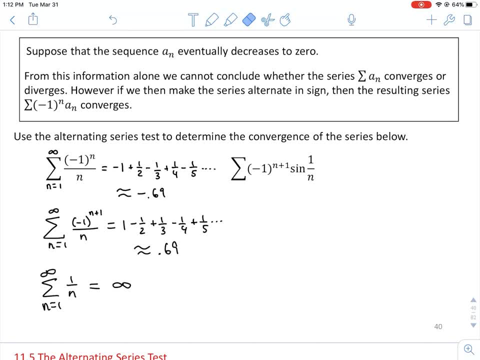 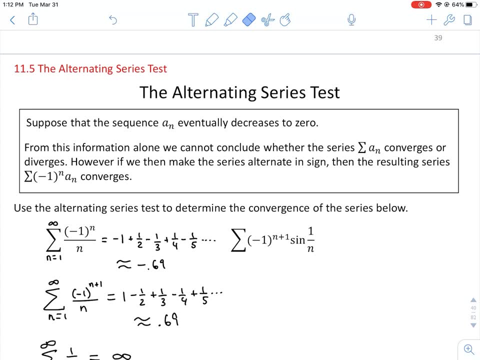 zero and then you make the terms also alternate in sign that the resulting series will always be convergent, And this is what the alternating series test says. Suppose you have some sort of sequence that eventually turns into a convergent and you have a convergent number. Suppose you have 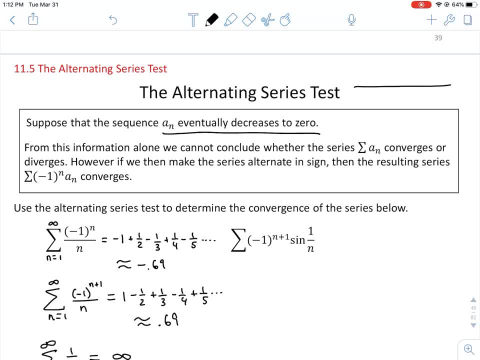 some sort of sequence that eventually turns into a convergent number and you have a convergent number eventually decreases to zero. To eventually decrease to zero means that so you have terms that maybe are all over the place, but eventually they get to a point where they decrease to zero. 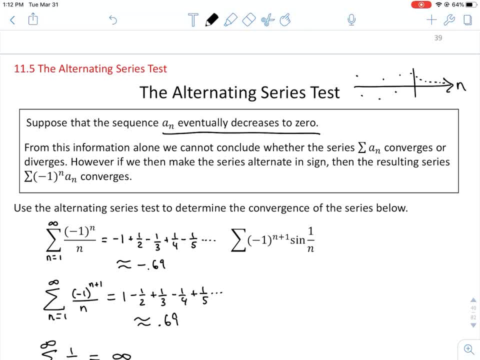 That also suggests that the terms eventually have to become positive and stay positive, because the only way you can decrease to zero is to be positive. If you have such a sequence, then we've already been able to show that the series is inconclusive. It's either divergent. 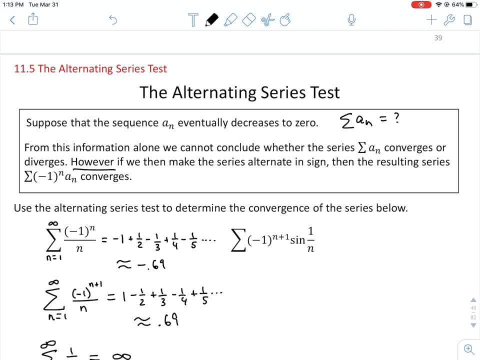 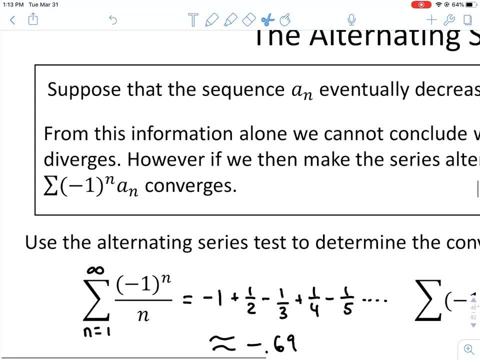 or convergent. We need more information, We need to do a test. However, if we make the series alternate in sign, then the resulting series will converge. Now, in my notes here, I only made it alternate in sign one way, by putting negative one to the n in front. but you can also conclude here: 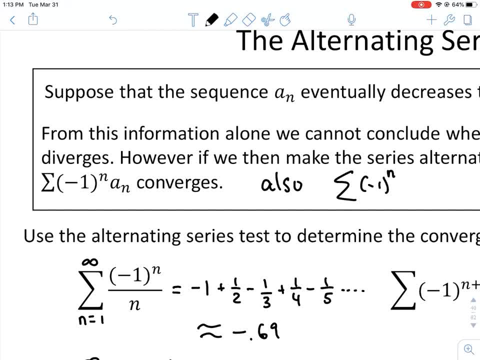 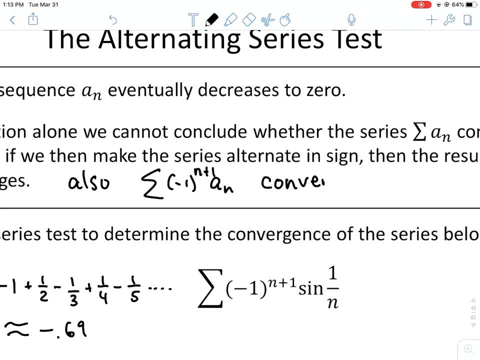 that if you make it alternate in the other way, the negative one to the offset by one. so we switch to where the pluses and minuses are, that this one converges as well. So you've got to make it alternate some way. Now, what's nice about the alternating series test is that students are 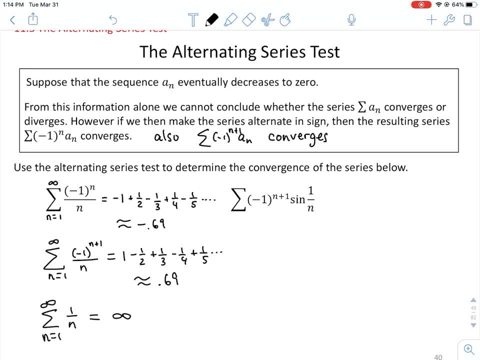 already tempted to say that if a sequence has terms that shrink to zero, then the series is convergent. Now, that's a faulty line of reasoning. What's nice about the alternating series test is that if a sequence has terms that shrink to zero and you make it alternate. 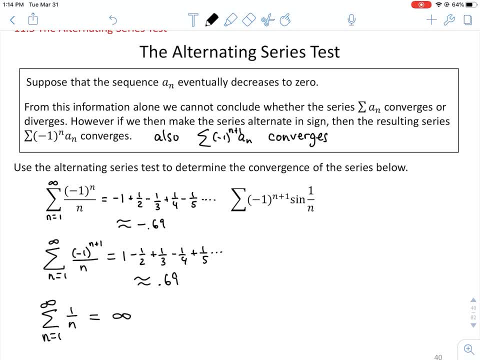 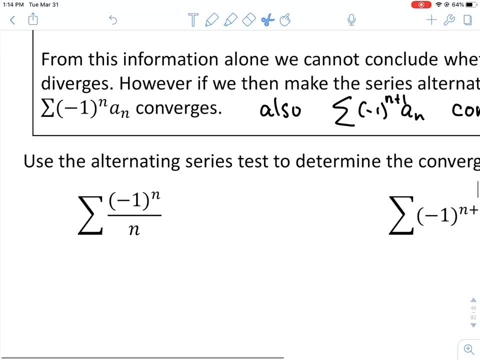 then yes, we can now say that the series will be convergent. All right, what this looks like. let me delete all this build up here. When you're looking at a series and you're trying to determine whether it's convergent or divergent and you notice that there's an alternating component, 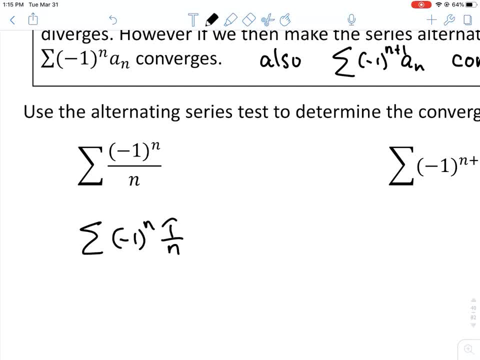 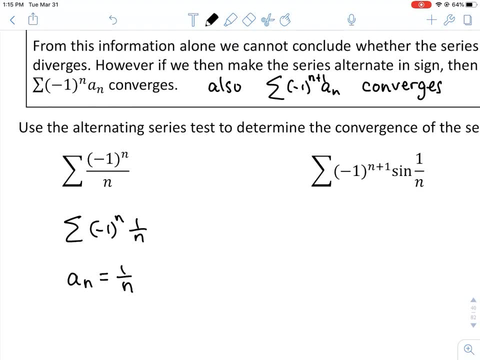 sometimes it's a good idea to separate the alternating component. Here is the a sub n that's referred to in this theorem, So the part without the alternating sign. And ask yourself: is this a sequence that decreases to zero? eventually, The answer to this is yes. 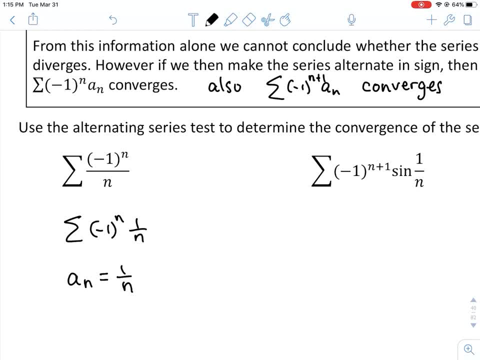 because the first term is one, the second term is a half. So this one's decreasing to zero from the get-go. It doesn't dance around and then decrease to zero. It decreases to zero right from the start, But all we have to do is say that this decreases to zero. Thus, when you do a series, 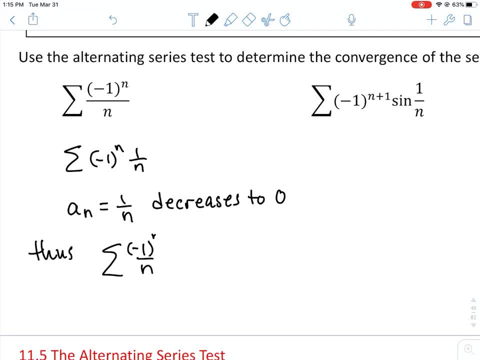 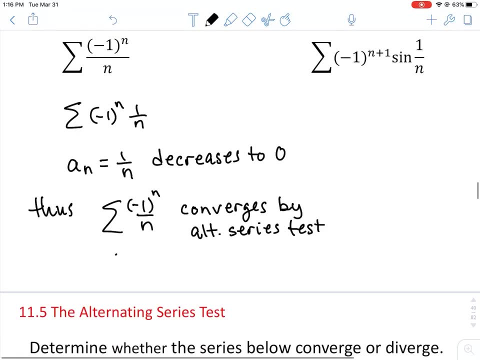 of it. now, this alone would be inconclusive, But if you make it also alternate, in some ways this series converges by the alternating series test And then using technology, we knew that this particular series, if you started at n, equals one anyway- was approximately negative. 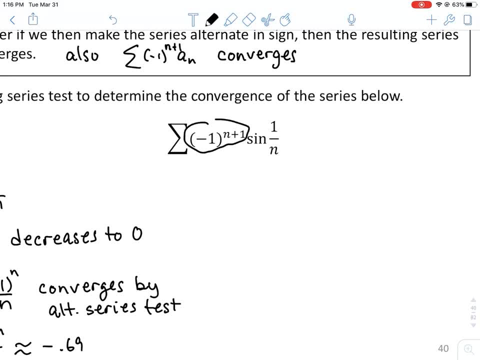 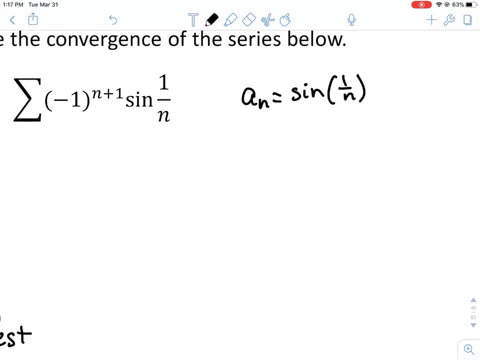 0.69.. All right, in this second example here, there's definitely an alternating component here, And so this is the sequence a sub n. we want to focus on in our analysis and ask ourselves what happens to it as n approaches infinity. Does this become a sequence that decreases to zero? 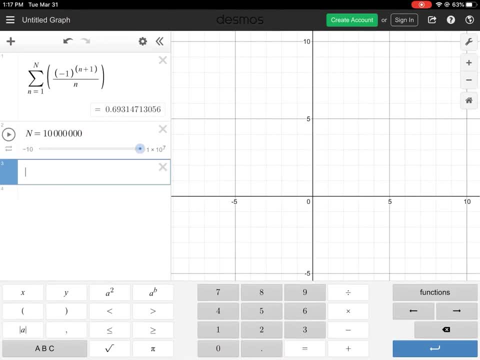 Well, you could answer this by going to Desmos And graphing the continuous function version of this, for y equals sine of one over, and then we're using x instead of n to graph a continuous function version. We have all sorts of craziness. 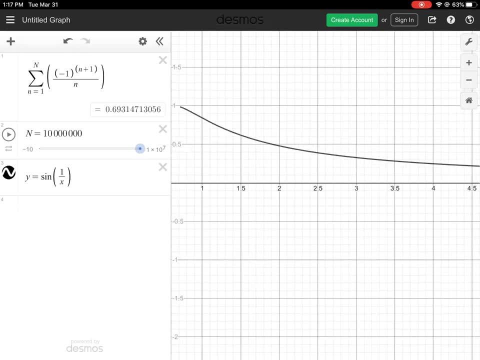 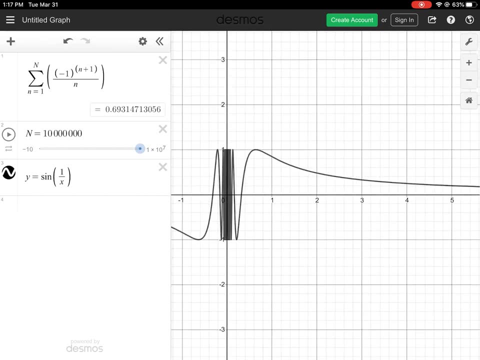 happening here near zero, but we're only interested in what happens as we go this direction. And as we go this way, notice that we do get a function that decreases to zero. So, in other words, the sequence would decrease to zero as well. The sequence would just be a bunch of points along. 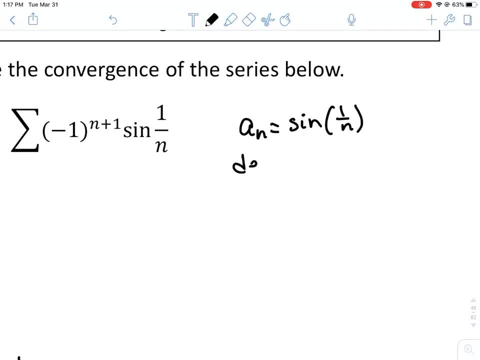 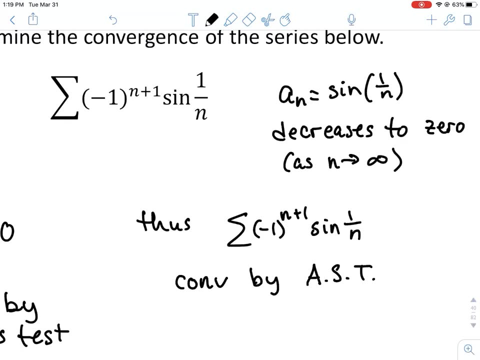 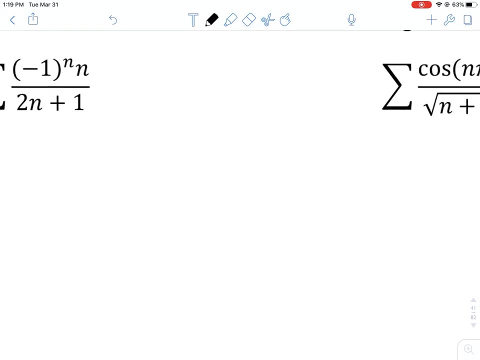 that curve instead of the continuous version. We know that this decreases to zero as n gets large, Thus converges by, and then a st will be my lazy way of saying alternating series. test The next slide. determine whether the series below, whether they converge or diverge. 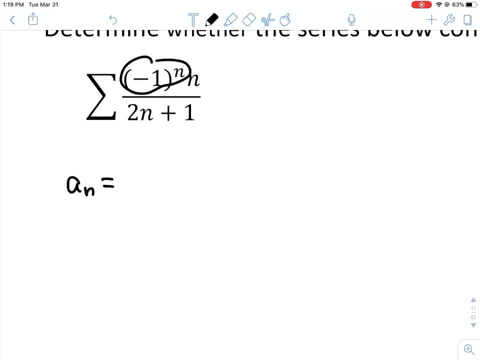 Now let's extract the a sub n, So get rid of the alternation. Okay, so get rid of that part and look at what's left. And our sequence in question is this: As n goes to infinity, this is a balanced rational function, So you can divide the leading coefficients. 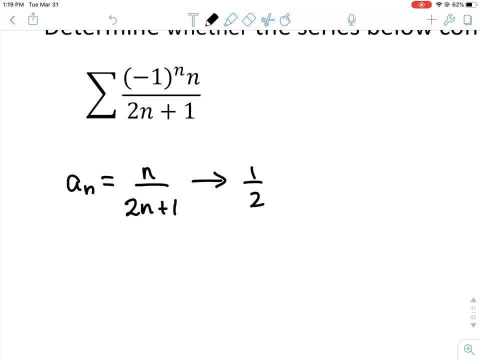 or you can use L'Hopital's rule here. But it approaches one half And right away, even though there's alternating signs here, we're going to get a series that decreases to zero. So we're going to see that this series has no chance of converging, because the sequence is converging to something. 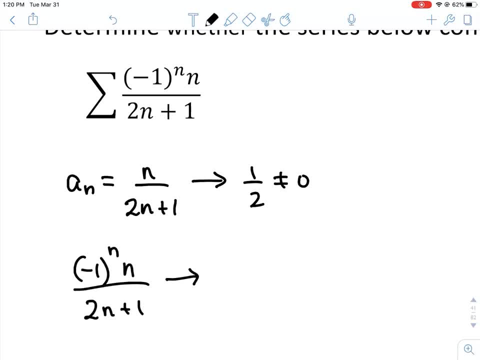 that's not zero. Even with the alternating sign, this is approaching what's not approaching zero. In fact, it's not approaching anything. It's approaching one half, then negative a half, then one half, then negative one half. Thus the series diverges by the divergence test. 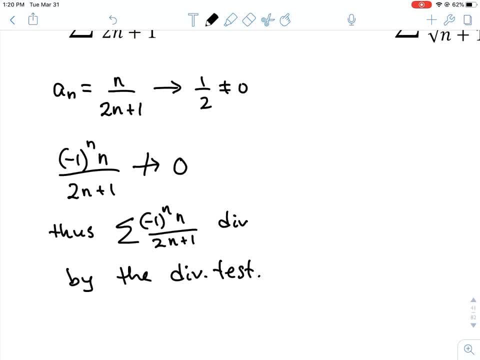 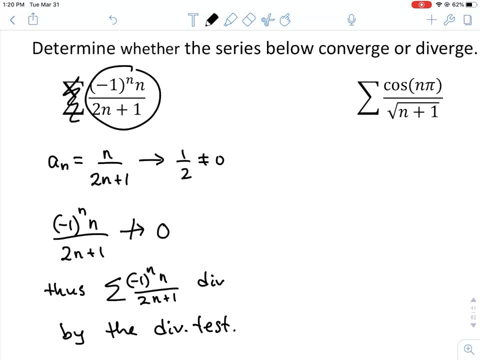 That was one of the first tests that we talked about. The divergence test is one of the first tests you should always scan is: just look at the sequence. Ignore the series. look at the sequence. if the sequence does not approach zero, then the series is always divergent. It's only when the 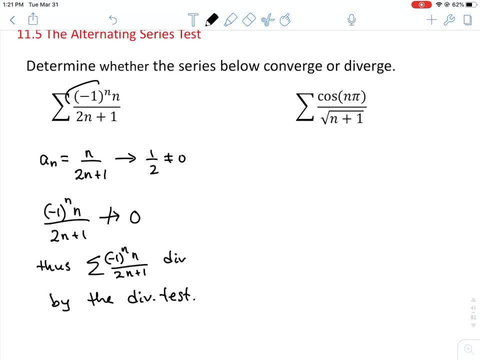 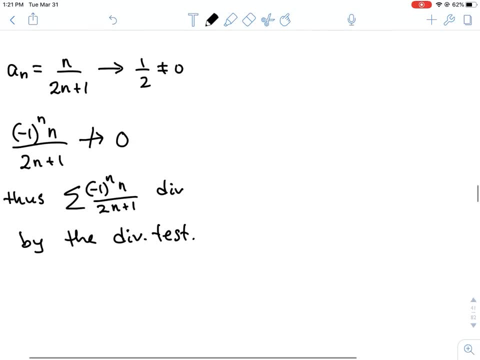 sequence does approach zero that we have to then do some other tests, Even though this is an alternating series. here I'm actually using a different test, the divergence test, to show that the series is divergent. You should never, ever, write a statement that reads: diverges by the. 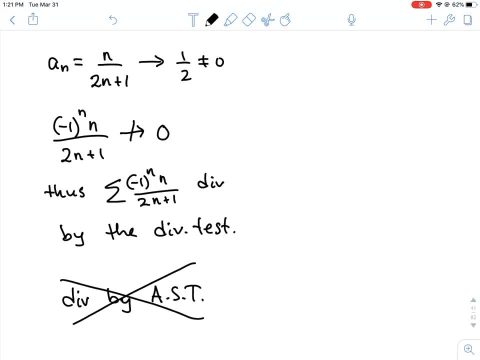 alternating series test. This is a bad statement. The alternating series test is not a test that shows divergence. It's a test that shows convergence, And if it fails to show convergence, then you need to use a different test to make a conclusion about your series. 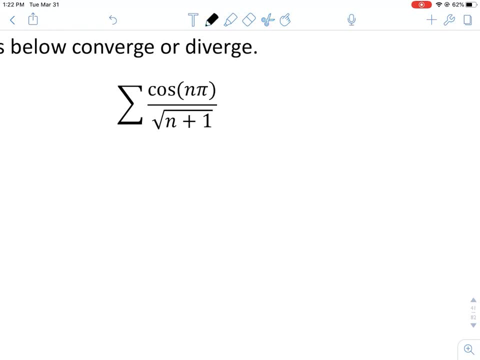 This next one here. it's an alternating series, but it's one that's in disguise. Let's take a quick peek at what this means up here. Let's just analyze this as a sequence. Let's start at n equals one and just get some terms. So when n is one, we get cosine of pi. 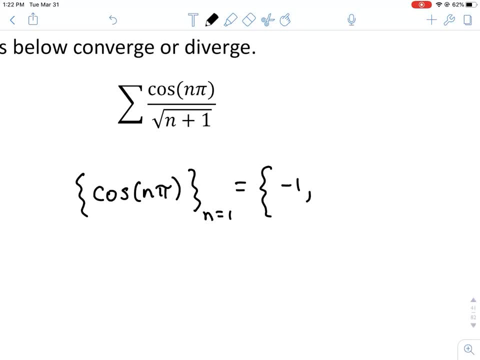 Cosine of pi is negative one. When n is two, we get cosine of two pi. Cosine of two pi is one. Plug in three. Cosine of three pi is negative one again. Notice that this is just a clever way to do. 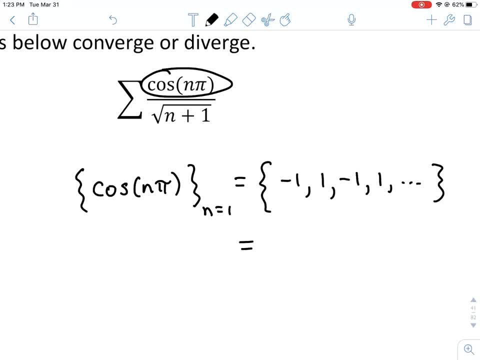 this. So if we see a cosine of n pi, we could just recognize that this is the same thing as doing negative one to the n right. Just verify that When n is one, we get this term, When n is two. 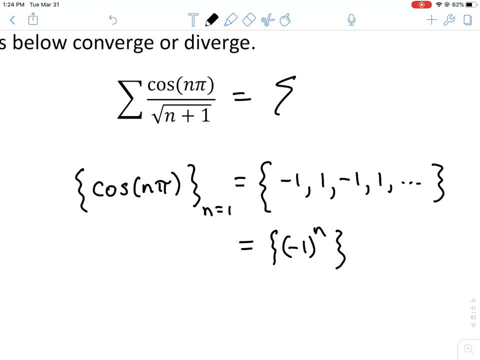 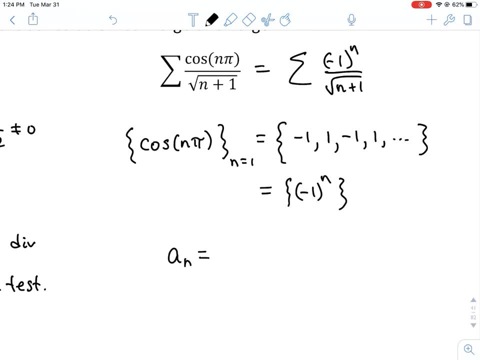 we get that. When n is three, we get that, et cetera. So I could rewrite this series up top as the series of just negative one to the n over radical, n plus one. But grab now the part that doesn't involve the alternation. So our sequence that we're looking at is one over radical, n plus. 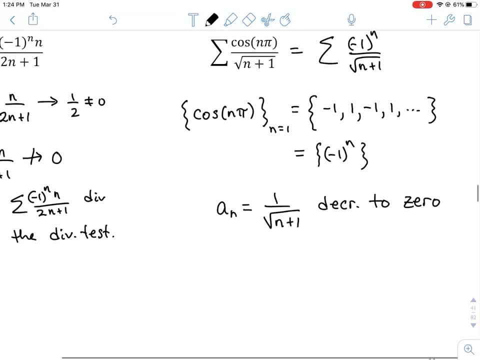 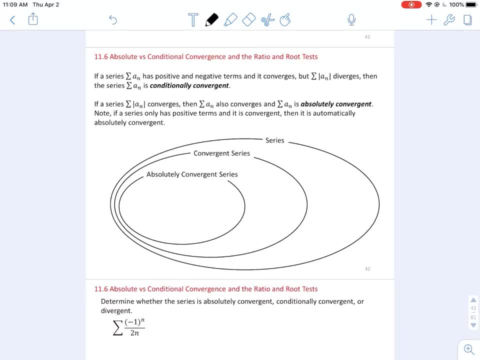 one. This does decrease to zero. This is what we need for convergence of the alternating series. I can use the alternating series test to conclude that this converges. Before we jump into what you're seeing here, let's just take a quick step back: The p-series test. If you look back at this slide here, 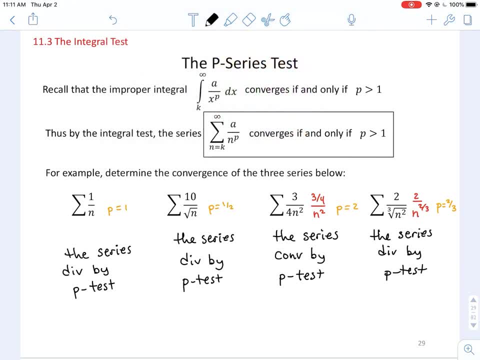 there were four series that were given. They were all p-series. Only one of them the power was large enough for the series to be convergent. That was this one. here The power was two, That's more than one, so that series was convergent. The other three were divergent series, because the value of p 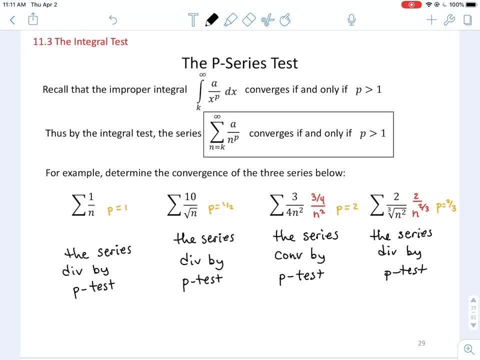 was small. Now, if you look at the sequences of all of these things, if you ignore this series here, as a sequence, that is a convergent sequence, It decreases to zero. Yet when you put this sum on there, then it becomes a divergent series. The terms will add to infinity. Same is. 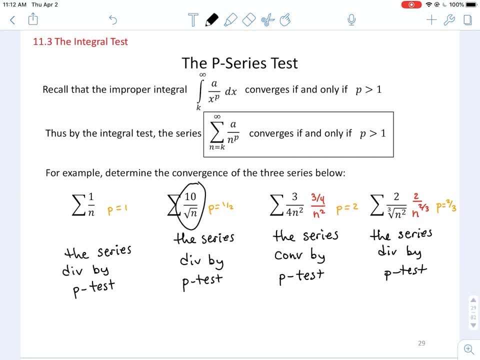 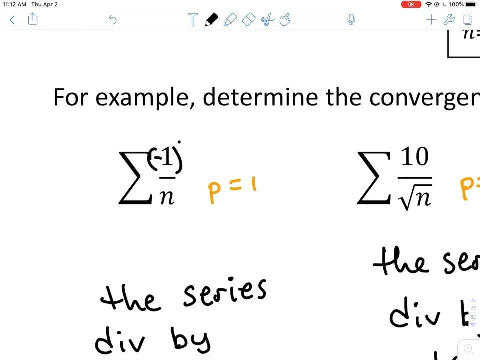 true for the other. This sequence is convergent. Its terms decrease to zero, but this series is divergent. The same thing is going to happen over here. However, if you take any of these divergent series and you simply make them alternate, throw a little negative in front of there with a power. 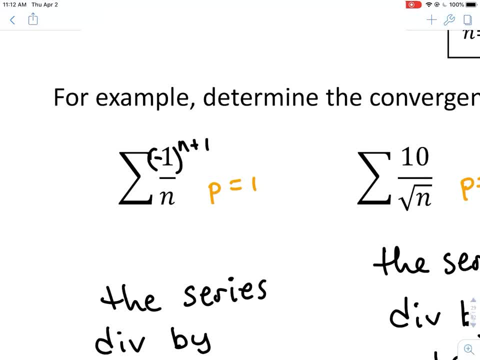 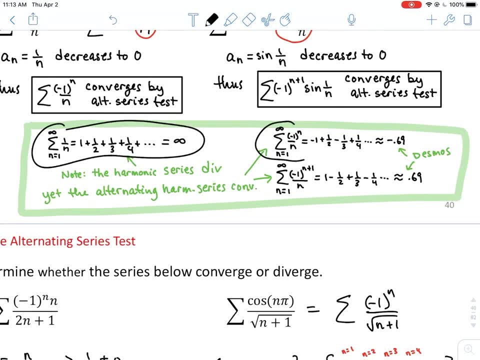 either n or n plus one. all of a sudden we'll have a convergent series. All right, so it's possible for a series to be divergent. yet when you make some of the terms negative- in fact every other term negative- it becomes convergent. This introduces a whole new way to categorize. 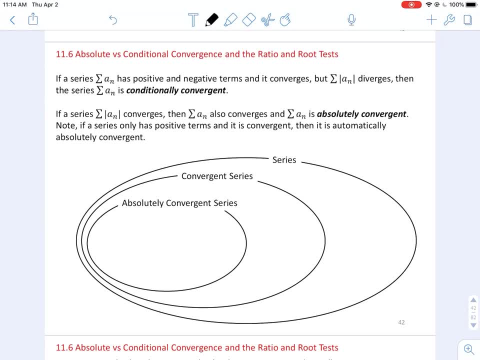 series into different classes. Hence, if a series has positive and negative terms and it converges, then it's convergent. But when you do the absolute value of all the terms, in other words get rid of all the negatives, make it only positives now and that series diverges. 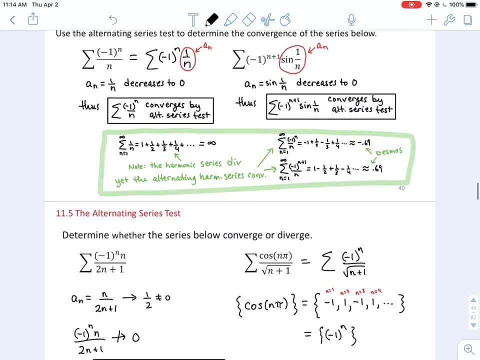 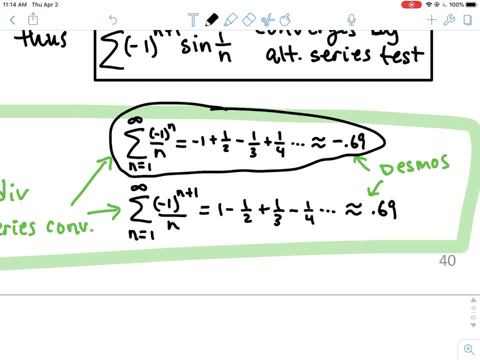 then the original series is said to be conditionally convergent. So our first good example of that is a harmonic series. So here's a series that has positive and negative terms right here and it's convergent. It adds to roughly negative 0.69.. Here's a second example. 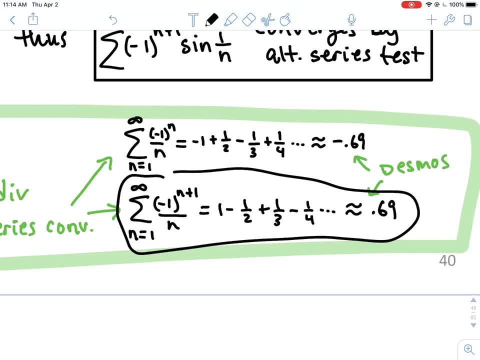 Here's a series that has positive and negative terms. convergent adds to around positive 0.69.. However, if you were to take the absolute value of this- in other words, get rid of the alternation, make them all positive- you would effectively turn. 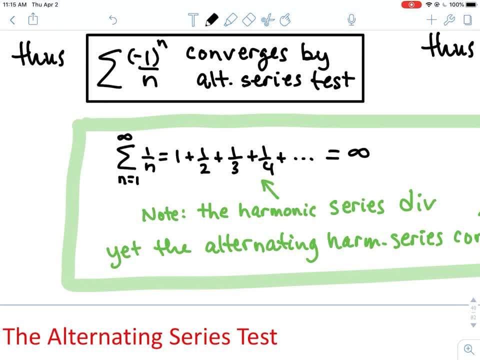 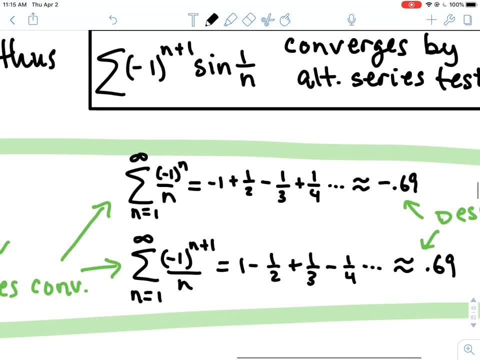 either one of these series into this one and this one is divergent. So in other words, the negatives have to be there to have convergence. So if you get rid of the negatives it becomes a divergent series. Therefore, these two series are said to be conditionally convergent. 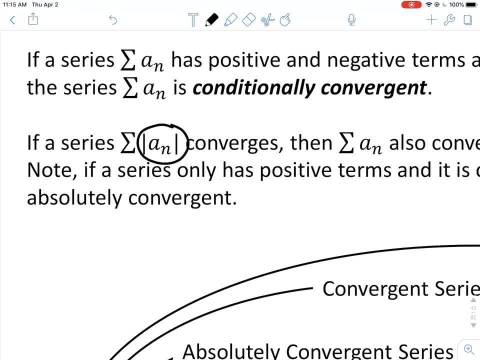 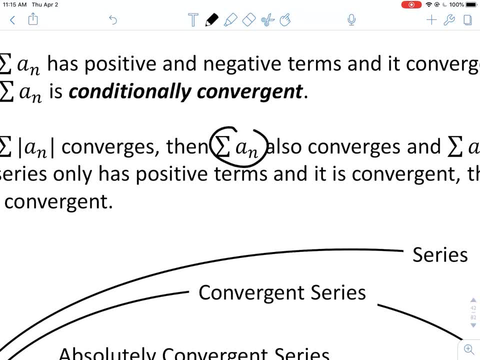 Now, if a series of the absolute value of terms of a sequence converges, it'll also be true that if you get rid of the absolute value, that the series without the absolute value- so maybe some of the negatives will come back- will also be convergent. 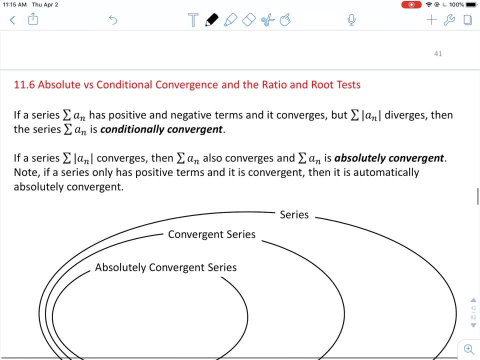 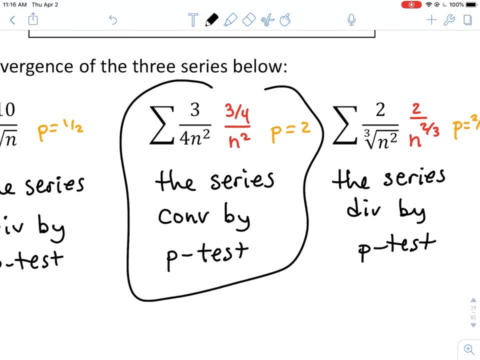 And we say that that series is absolutely convergent. It'll converge with or without the minus signs. Let's look at that one p-series that was convergent already. This one is convergent and it's only positive terms. But if I did put a negative 1 to the n on here and made this also, 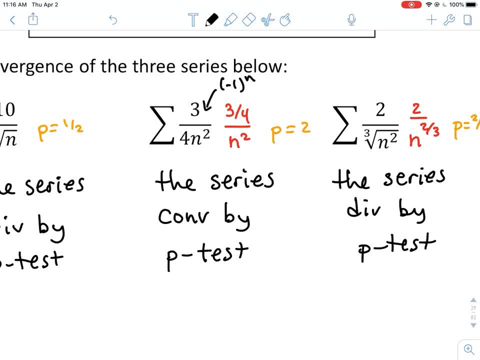 alternate, it would also still converge. It would converge by the alternating series test. But if I looked at with only positive terms, it would still converge. So we say that this is an absolutely convergent series here. With or without the alternation, it would still be called. 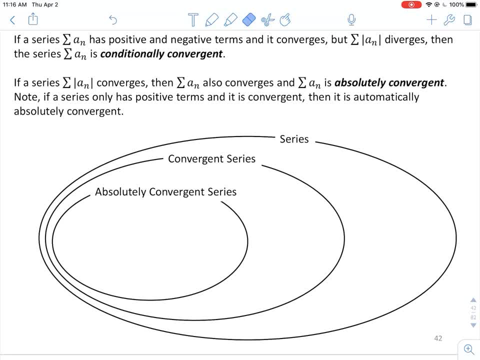 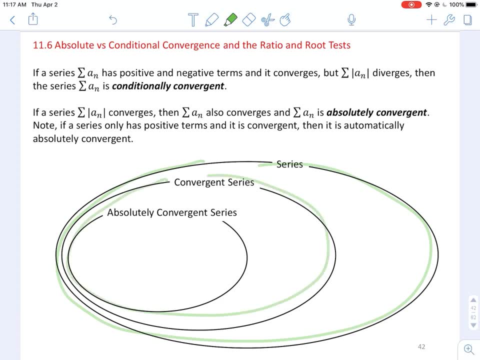 absolutely convergent. Okay, so we have this Venn diagram that we have Biggest circle here is just all series. And then we have convergent series is a smaller subset And then absolutely convergent series is an even smaller subset. So let's go ahead and put some examples in here. Let's first 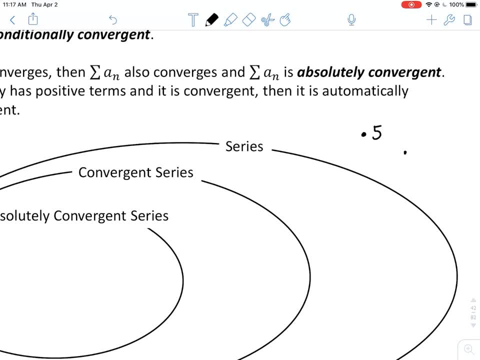 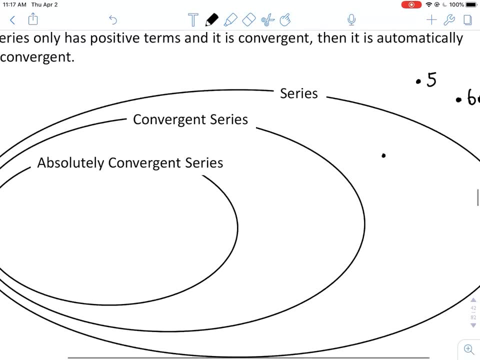 do an example of something that's not a series. Just the number five is not a series. Something, even a number- A brick- is not a series. All right, then the example of something that is a series, but because it's outside of this circle, it has to be a divergent series. So there's lots of 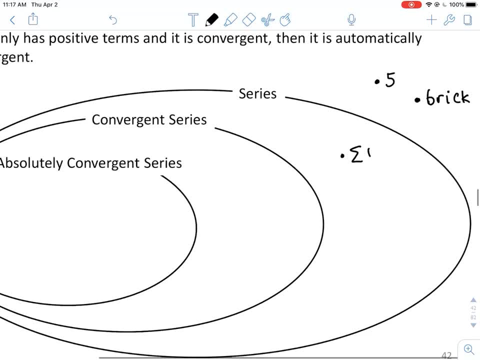 different divergent series. We can add up ones forever. That would be divergent. We can add up n forever, In other words, 1 plus 2 plus 3 plus 4, that adds to infinity. That's divergent. 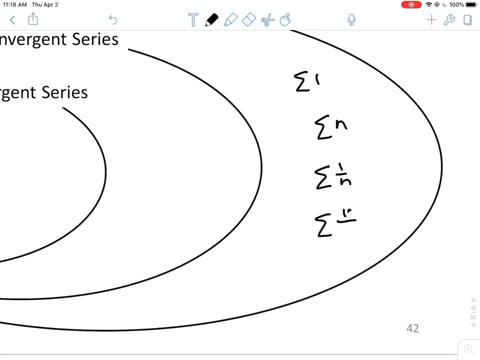 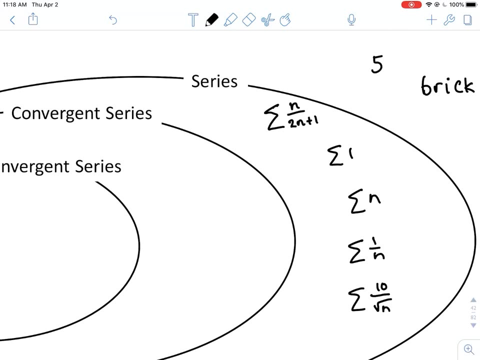 So you have the harmonic series or other kinds of p-series- 10 over rad n- right? This is a p-series. The power is one half. It's not big enough, right? All of these things are divergent series. Another example: let's do an example of n over 2n plus 1. This is a divergent series because 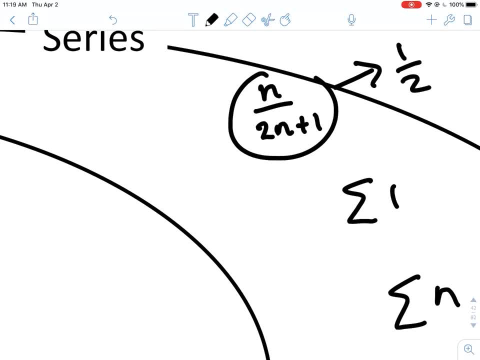 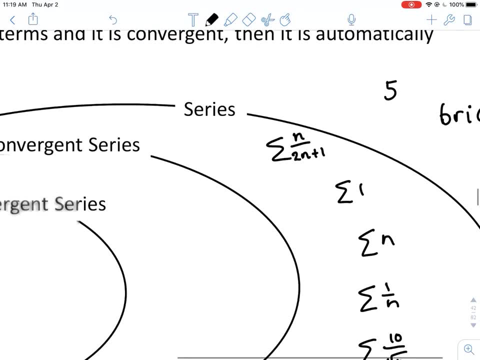 as a sequence, this approaches one half, So it's a convergent sequence. However, if you then try to add up all the terms, it's like adding up one half forever, which adds to infinity. So this is clearly a divergent series. Now we want to start listing some series that are convergent but that. 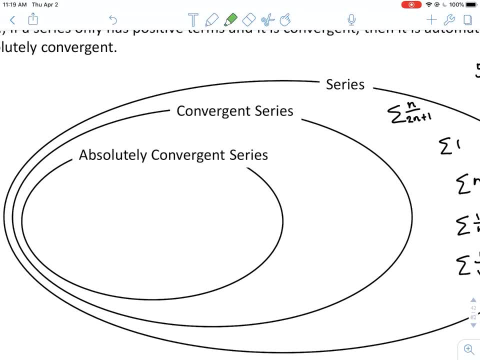 are only conditionally convergent. So the conditionally convergent a window here is pretty much anything inside the convergent but outside the absolutely convergent. This space here is where the conditionally convergent series reside. So let's do some examples of those. The first one we did was that alternating harmonic series. This is a 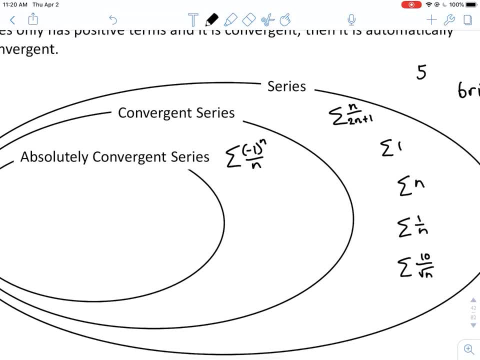 series that converges And to be conditionally convergent- you might have started to sense this already- there has to be negative terms involved. Because if there are no negative terms involved, then the series is either just absolutely convergent or it's divergent Pretty much. 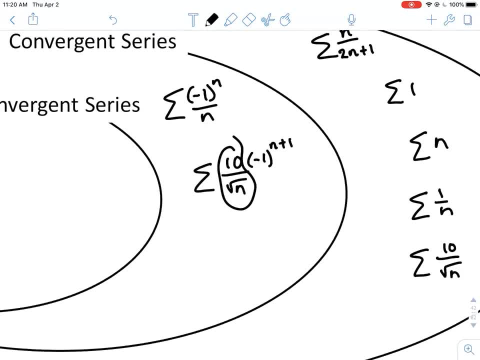 everything is convergent. So the conditionally convergent series is pretty much write down any p series where the power is one or less, but it still has to be a sequence that goes to zero. So this, the thing I just circled, that does go to zero. If it goes to zero and you make it alternate and then 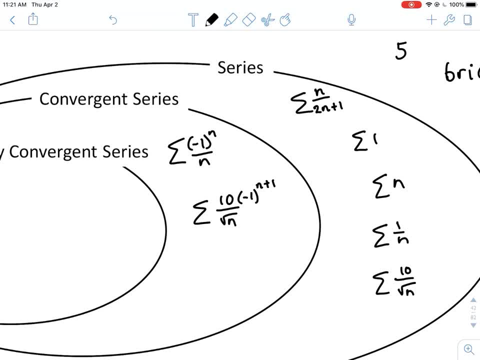 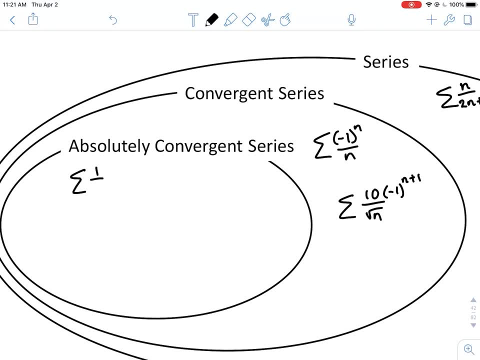 you add them all up, you will get a convergent series. So these are some examples of some conditionally convergent. Get rid of the alternation and they become divergent And then absolutely convergent. there is a series of only positive terms. but by the p-test this is a convergent series and it's only positive terms. 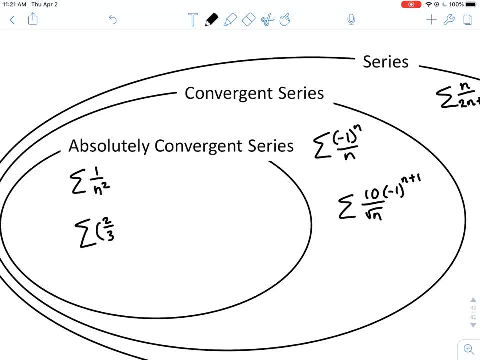 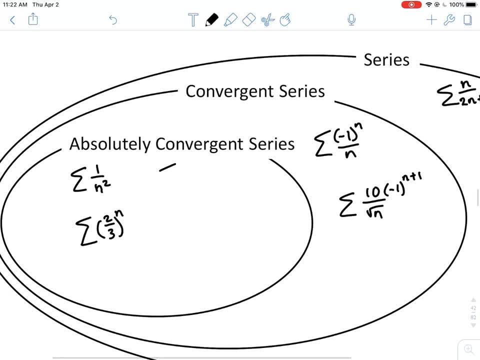 A geometric series that converges Something like two-thirds, which is my ratio. raise that to the end. This is convergent because the ratio is between negative one and one. You can also do some terms that have negatives, Do an alternating p-series where the power p is more than one. 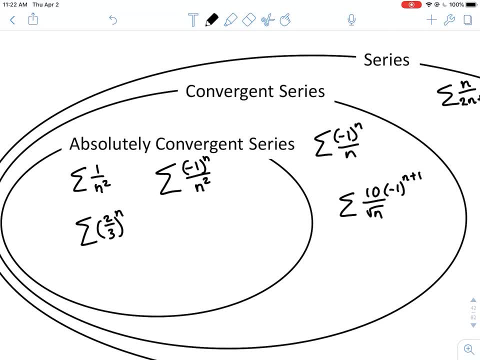 This is convergent the way it's written, but it would also be convergent if you got rid of the alternation. In other words, if you turn it back into this one, With or without alternation, the series converges. Therefore, we say it's an absolutely convergent series. both of these, That's absolutely convergent and that's absolutely convergent. 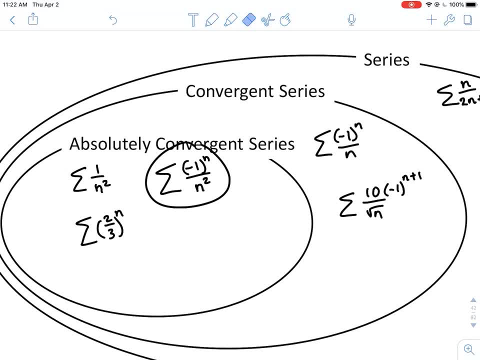 Sometimes people think that in order to be absolutely convergent, you can only have positive terms. but no, no, you can have negative terms involved and still be absolutely convergent. You can even have a- let's do a negative three-fourths ratio. So let's do a geometric series that also alternates, but its ratio is between negative one and one. 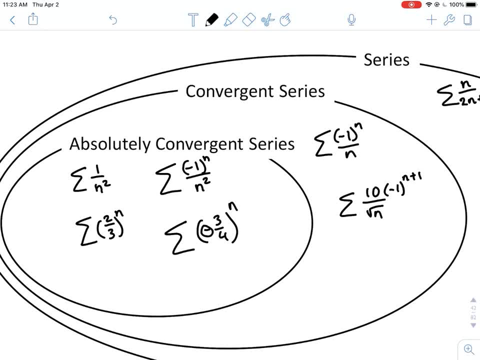 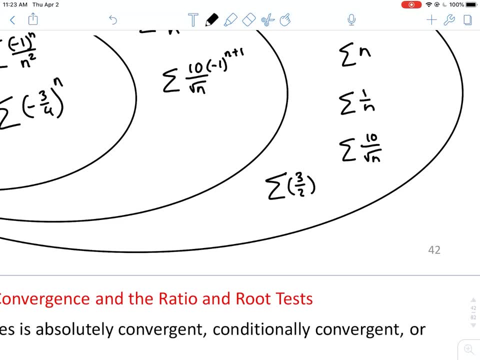 Therefore it will converge, Get rid of the negative and make it only positive terms, and it still converges. So it's absolutely convergent, Whereas if you had a geometric series where the ratio was more than one, like three-halves, that's going to be divergent. 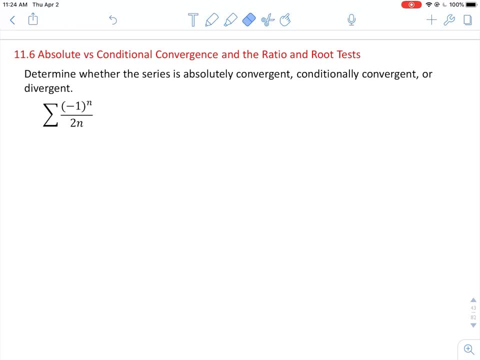 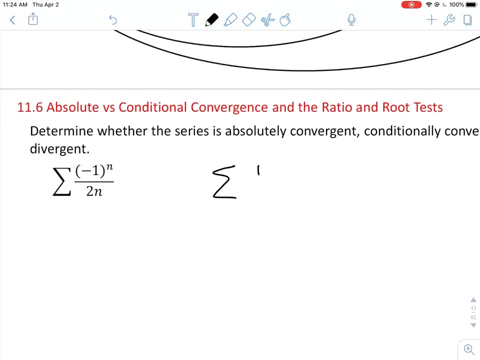 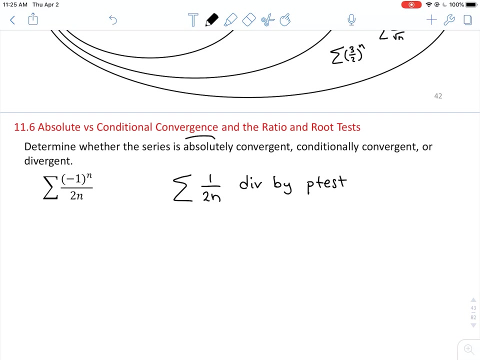 Determine whether the series is absolutely convergent, conditionally convergent, or divergent. Now, the way to test this is to go straight to the series without the negatives. Consider this series right here. This is divergent p-test. Now, if you got rid of the negatives and the result was convergent, then we're done. We say that the absolutely convergent would be the answer. 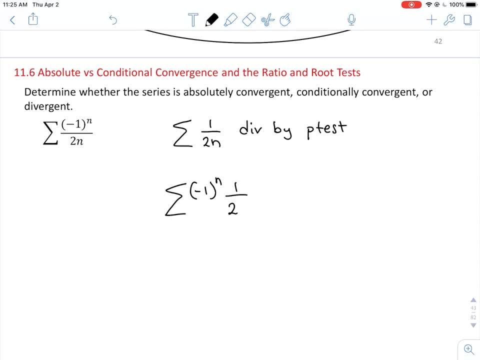 Now we've got to see whether it converges the way it's written. You could write it this way too, just sort of pull the alternation off to the side, so you can grab just this part here as a sequence, not as a series, mind you. 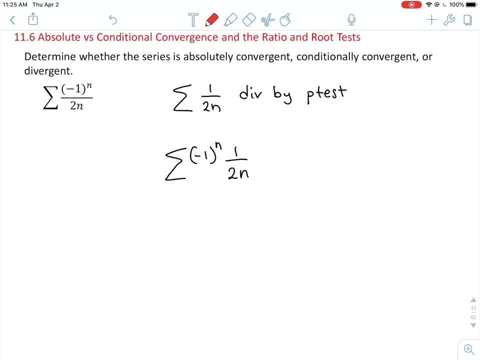 We're now thinking sequence. Up here we were thinking series. That's why we said divergent, But as a sequence- 1 over 2n- this does decrease to 0 as a sequence. I'm going to emphasize that we're thinking sequence here by putting in curly brackets. 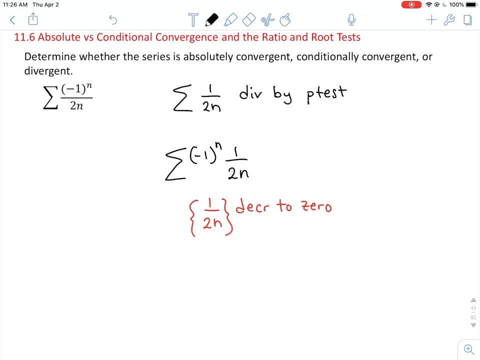 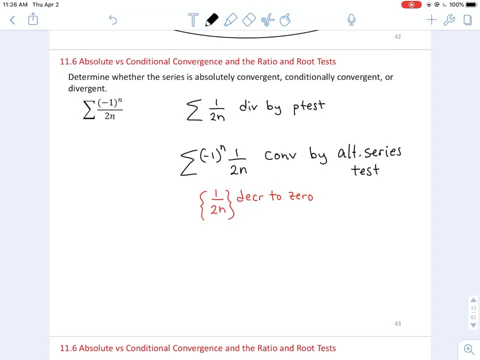 Therefore make the sequence alternate and then add them up, we get a convergent series. So this converges by the alternating series test, Because the series converges the way it's written, but get rid of the negatives and it then diverges. 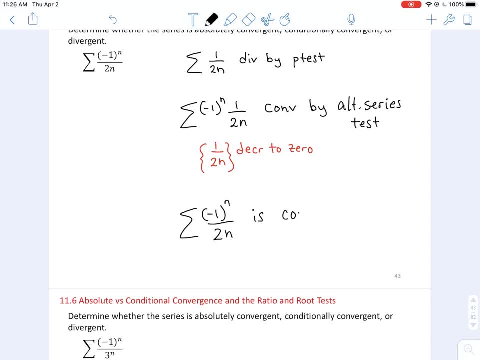 we then say that the original series converges by the alternating series test is conditionally convergent. Okay, let's look at the next one. This is actually a geometric series. You could use a little bit of properties of exponents and write it this way: 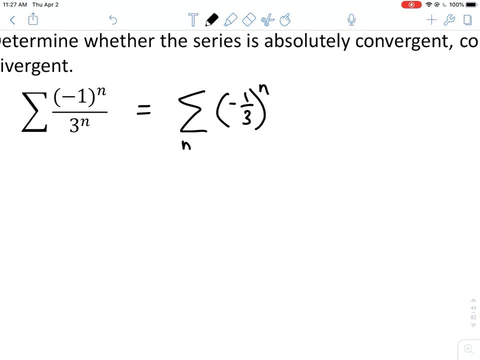 And this is a geometric series whose ratio is negative: 1- 3rd. For example, if we started at 1, the first term of this would be negative 1- 3rd. The next one would be positive 1- 9th. 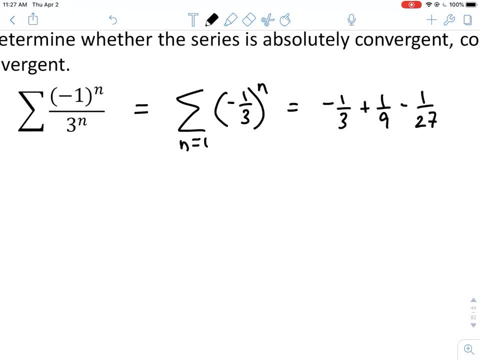 then negative 1- 27th, Right to go from term to term. we just multiply by negative 1- 3rd. So it doesn't really matter where it starts, but if it did start, it's easier to see that this is just geometric. 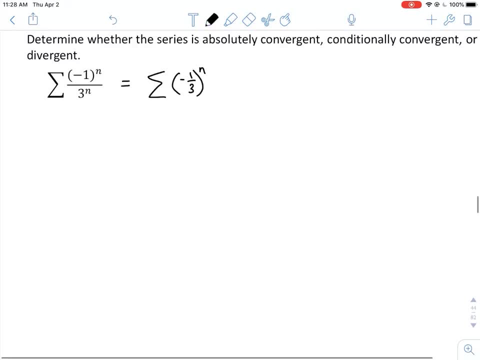 And because the ratio is between negative 1 and 1, this will converge. the way it's written, Let me do the absolute value of all the terms, In other words, just get rid of the alternation and reconsider. This is a convergent geometric series, right? 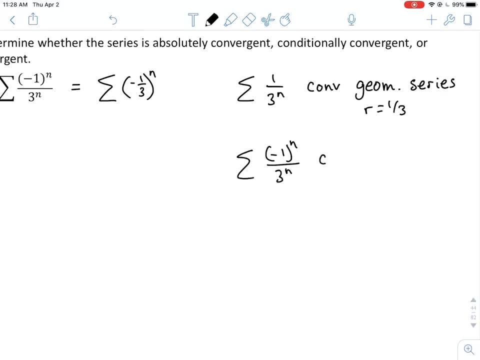 because the ratio is 1. 3rd, If you put the alternation back in, this is still a convergent geometric series. And remember, if the ratio is between negative 1 to 1, this is in the interval from negative 1 to 1.. 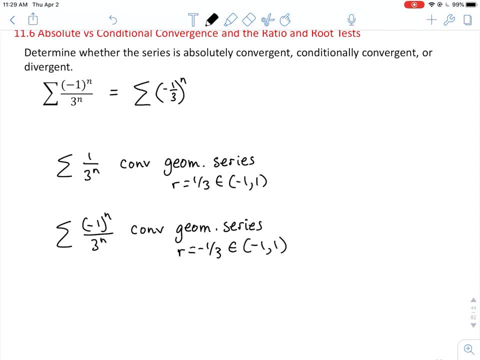 This is in the interval from negative 1 to 1.. So in both cases the series is convergent series. But really I just had to do this first step. Once I got rid of the alternation and I saw that it still converged. 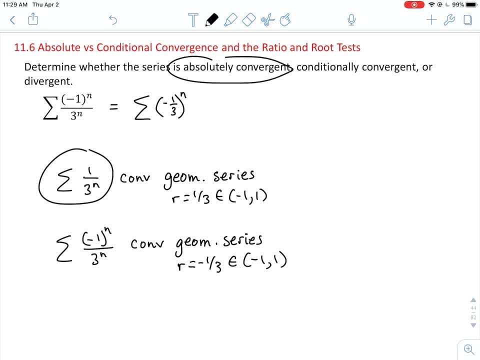 right away. I know that absolutely convergent is the correct answer. It won't be this and it won't be that, Which suggests that because it's absolutely convergent that it converges the way it's written With the negatives, it's still convergent. 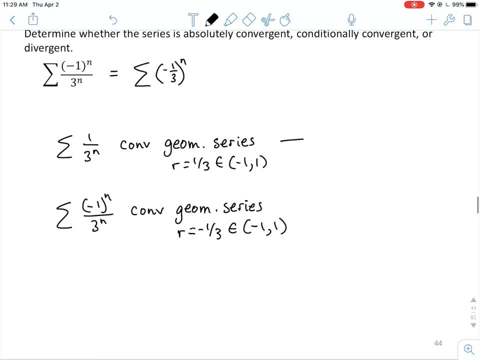 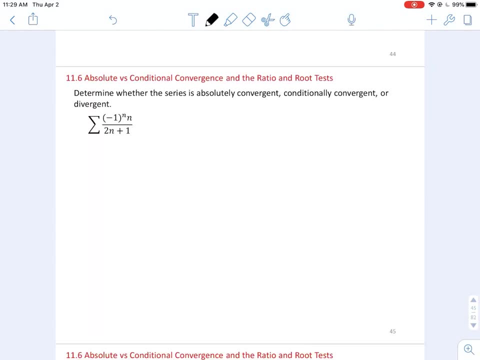 If it converges without the negatives, then it converges with the negatives. This first step alone was all I needed to know that the original series is absolutely convergent. Now here's an alternating series, So there's negatives again. So it's possible that's only conditionally convergent. 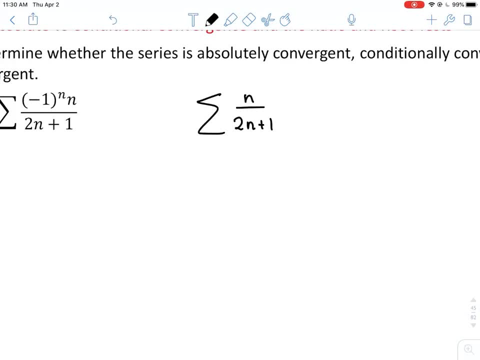 Get rid of the alternation. It's the first step. This sequence here approaches 1 half. Well, 1 half is not 0, right. In order for a series to be convergent, the sequence has to go to 0.. 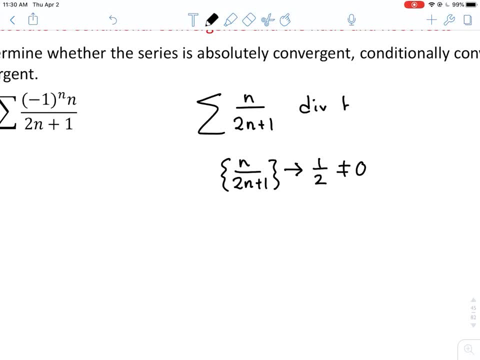 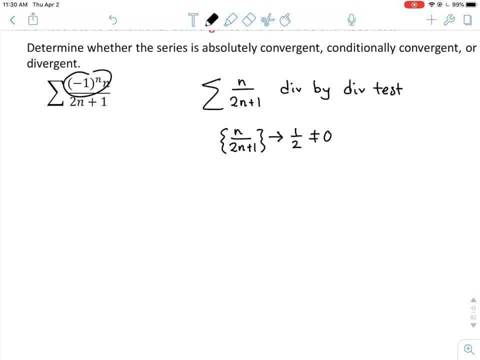 And since this sequence is going to 1 half, so this diverges by the divergence test, When I put the alternation back in, it's just going to make a sequence that approaches 1 half negative, 1 half, 1 half negative, 1 half. 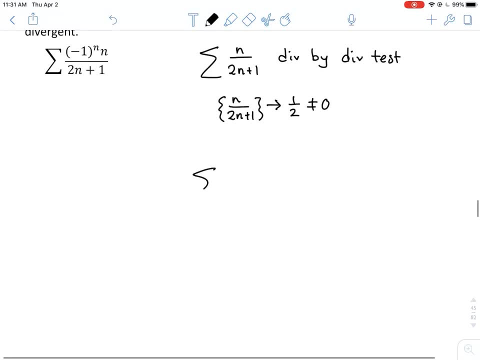 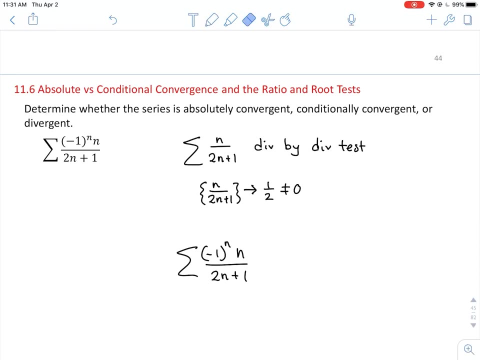 So even with the negative in place, the series is still divergent. Determining if it's obviously divergent first maybe is the best thing to do, And if it's not obviously divergent, then you can see if it's absolutely convergent, etc. 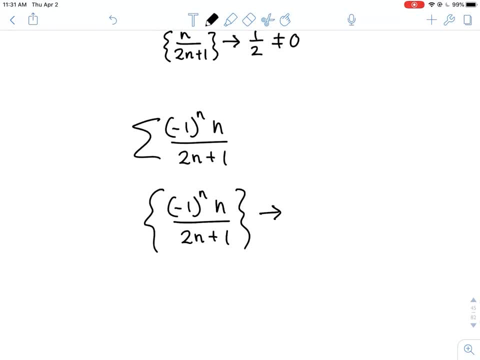 Anyway, put the negative back into play. But as a sequence this does not even approach a half. It has no limit. It approaches 1 half negative, 1 half, 1 half negative, 1 half. But to have a limit for a sequence? 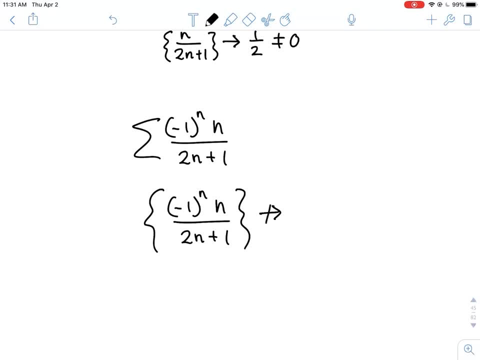 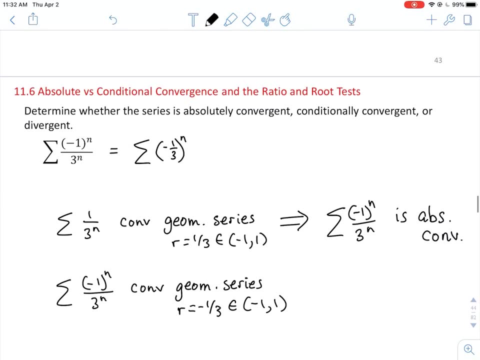 you have to approach a single number And this has no limit. Therefore it's not approaching 0.. Therefore the series diverges by the divergence test Of these options. I would pick divergent Up here. it was absolutely convergent.